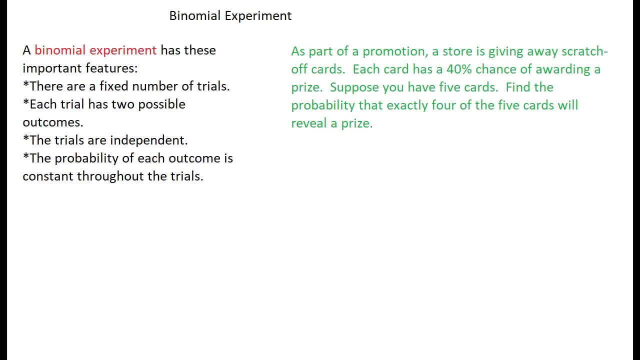 Hello. Today's video we are looking at a binomial experiment. A binomial experiment has these important features: There are a fixed number of trials. Each trial has two possible outcomes. The trials are independent and the probability of each outcome is constant throughout the trials. 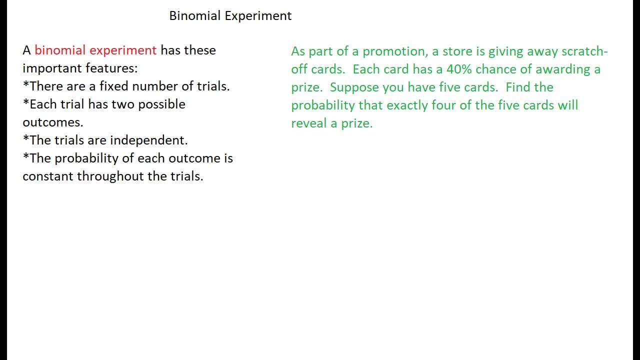 All right. Well, let's look at a problem and we'll see if this is a binomial experiment. As a part of a promotion, a store is given away scratch-off cards. Oh, I need to go to that store. Each card has a 40% chance of awarding a prize. Suppose you have five cards. Find the probability. 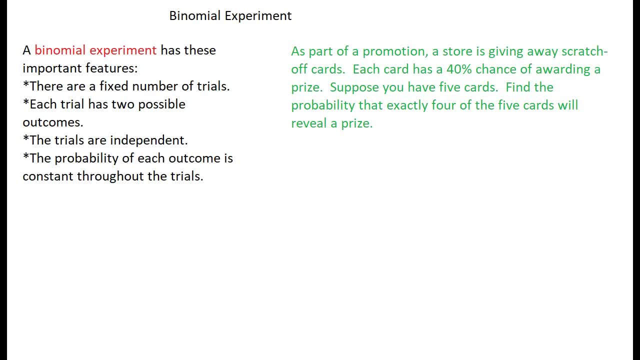 that exactly four of the five cards will reveal a prize. All right, Well, let's go through our checklist. There are a fixed number of trials, That is true. There are a fixed number of trials. True, The number of trials that we would have- and let's just call it N- is five, because you have 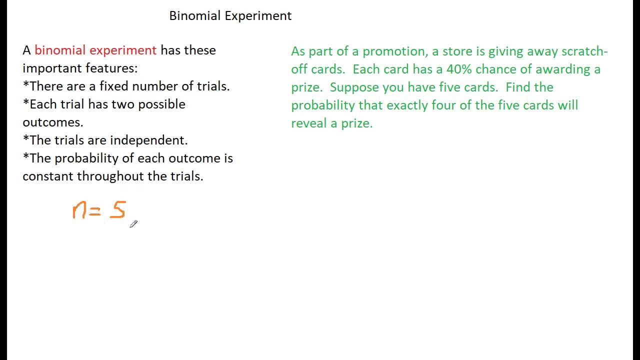 five cards, All right, And each trial has two possible outcomes. That's true too. You either win or you don't win, Right, So that works And the trials are independent. Well, yeah, If you scratch off one card and it's a winner, it does not mean the number of trials is independent. 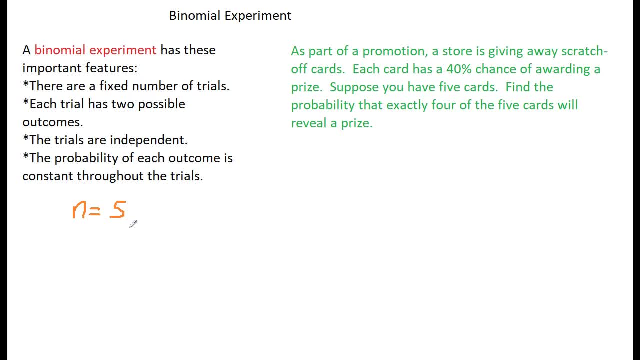 Next one will or will not. They do not depend on each other. So that is true, And the probability of each outcome is constant throughout the trials. Well, that's true. It says each card has a 40% chance of awarding a prize. All right, So let's go to it. We want to find out the probability that. 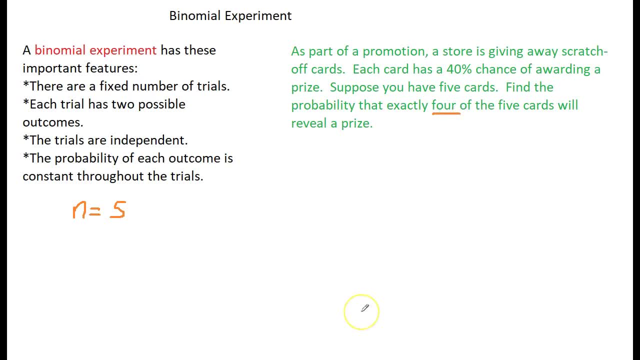 exactly four of the five cards will reveal a prize. All right, So let's go to it. We want to find out the probability that exactly four of the five cards will reveal a prize. All right, Now this is a combination. How do I know? The order doesn't matter, It does not matter which four. 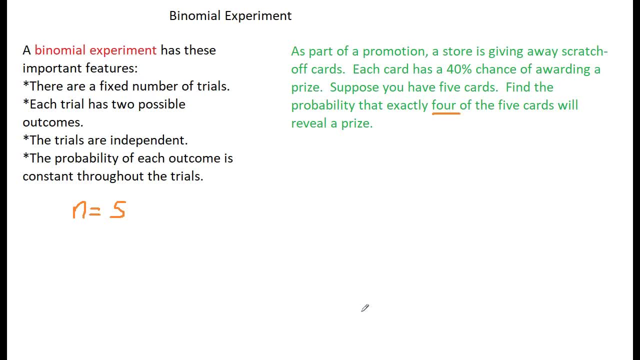 It doesn't say the first four, the last four or any combination of four like the first two and the last two. It doesn't give anything like that. So it's a combination. Order does not matter. Okay, So our N is five because we have five cards. X is going to be four. 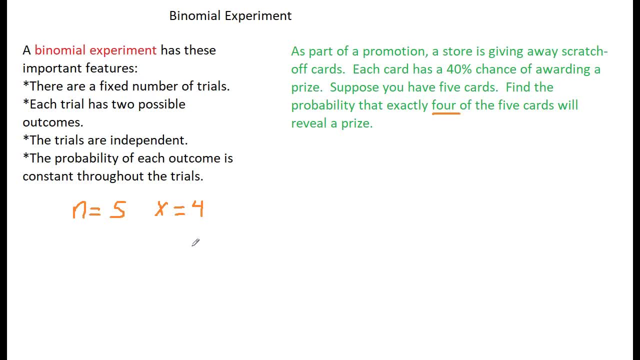 Because we want exactly four of the five cards to be winners. Oh, that would be nice, huh, Win some prizes. Now the probability, so probability P of a success that means a win is 40%. Now written as a decimal is 0.4.. Now the probability of failure: Q. 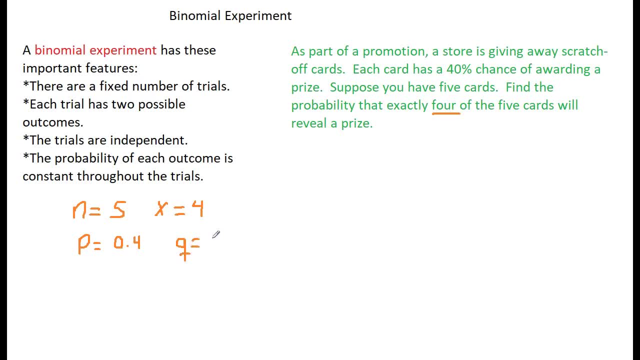 is 1 minus 0.4, which is 0.6.. Ooh, it looks like the odds are against us. All right, So the probability, all right, of X. here's our formula. Okay, Happening is this: It is N, C, X. 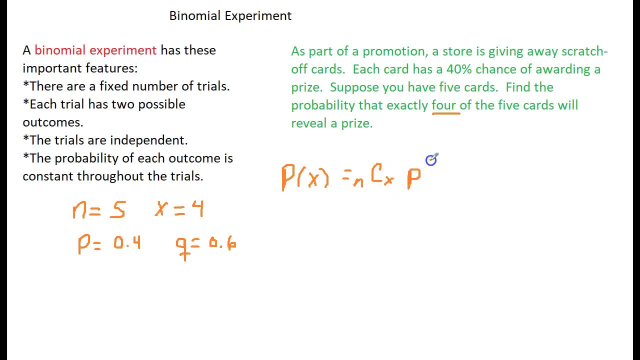 all right times P to the X power and Q times Q to the N minus X power. That is our formula. So now we are going to plug our values into this. So the probability of four winning cards in our scratch-off cards out of the five cards is five. 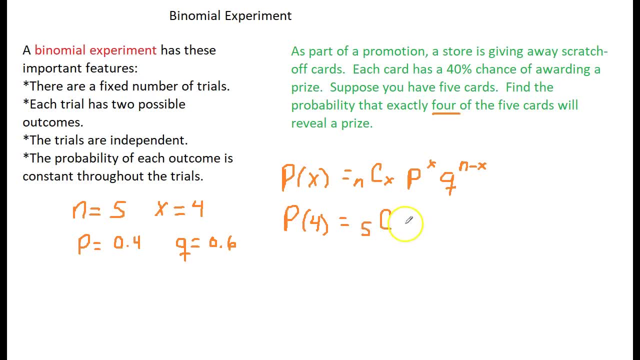 Five, C, four times 0.4, raised to the X power, Now what is X? X is four. So to the fourth power times Q, the. you know the probability of the loss. ooh, zero points. 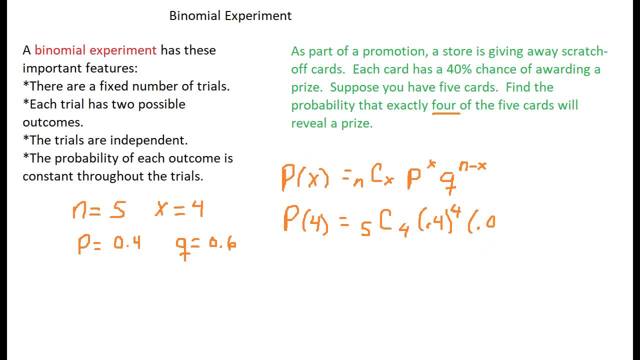 not point zero. Shame on me, I got points in the wrong spot. I got excited: Zero, point six or just point six. Let's just do point six. Now it is to the N minus X. So five minus four is one power. Okay, And so plugging this using our calculators. probability of